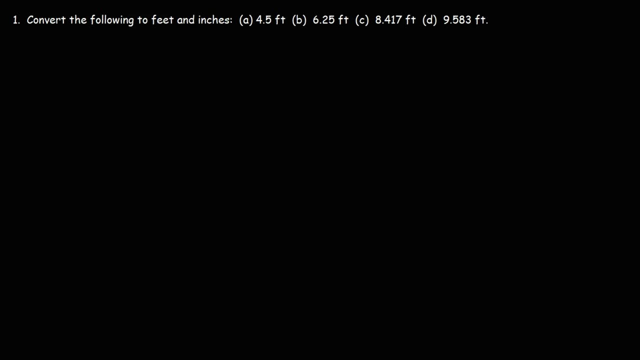 In this lesson we're going to talk about how to convert feet to feet and inches. So let's begin with part A. We have 4.5 feet. How can we convert that to feet and inches? Now, what you want to do is break this into two parts. 4.5 feet is 4 feet plus 0.5 feet. 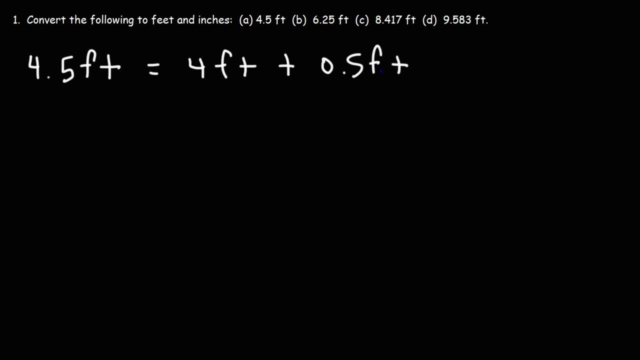 Thus we have 4.5.. Now the decimal portion, the 0.5, we want to convert that to inches, So we can write the conversion factor here. To convert feet to inches you need to multiply by 12.. 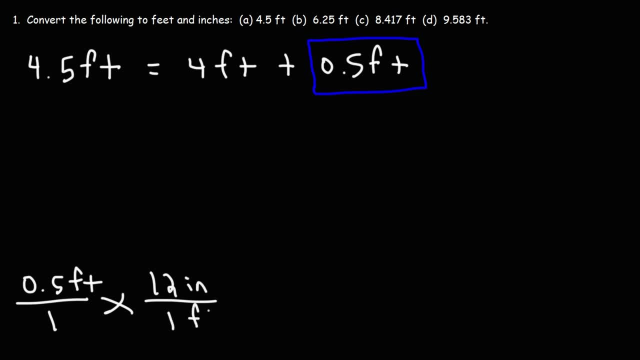 There's 12 inches in a foot, So I set up the conversion in such a way that the unit feet will cancel. So it's 0.5 times 12.. That gives us 6 inches, So we can write this as 4 feet and replace this with 6 inches. 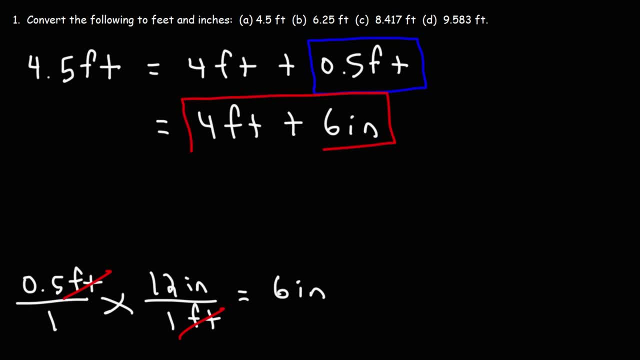 So that's what 4.5 feet is equivalent to. It's 4 feet and 6 inches. Try this example, part B: Convert 6.2 feet to inches. That gives us 0.25 feet to feet and inches. 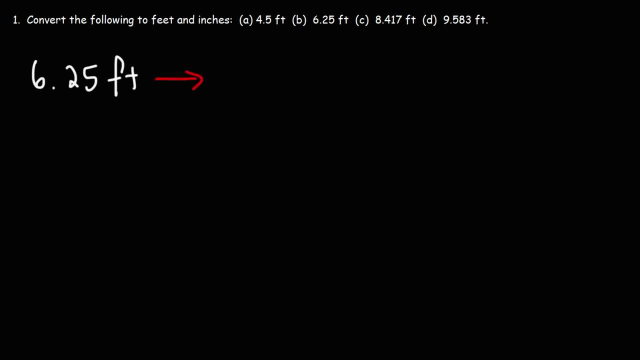 Feel free to pause the video, So let's break it up into two parts. This is 6 feet plus 0.25 feet, So let's convert this part- the decimal part, 0.25- to inches. We're going to follow the exact same process. 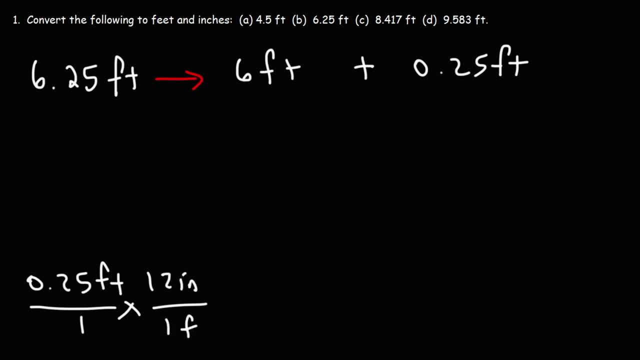 We're simply going to multiply it by 12.. 0.25 times 12. That is equal to a nice whole number, which is street. So 0.25 feet is street inches. So our original problem 6.25 feet. 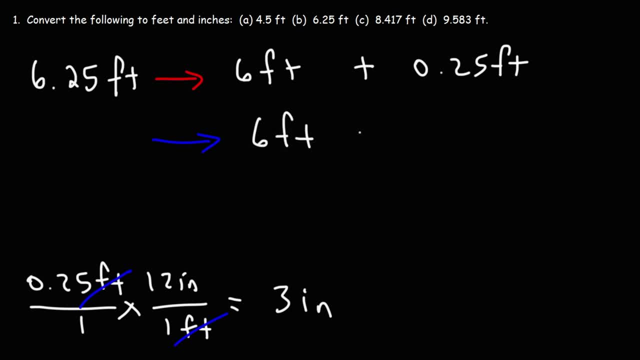 That's equivalent to 0.25 feet, So that's equivalent to 6 feet and 3 inches. We can also write it this way: 6 feet and 3 inches, And that's equal to 8 inches. Now, for the sake of practice, go ahead and try parts C and D. 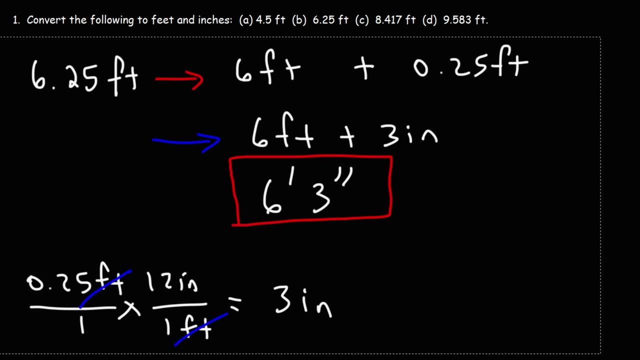 Aren't those two just the same thing? Very similar, Although they are the same. They're not just the same thing. They're just the same除 of Xu and D. They only grew a few shades in between the other parts at that time. 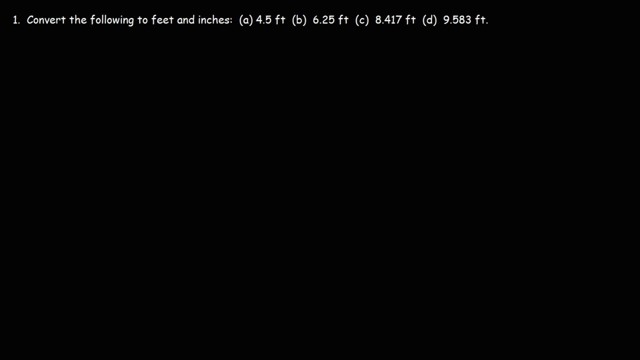 We've got two teachers here free to take a minute and work on those two examples, So let's start with part C. We have 8.417 feet. Let's break that to. let's break it into two parts, So we have 8 feet plus. 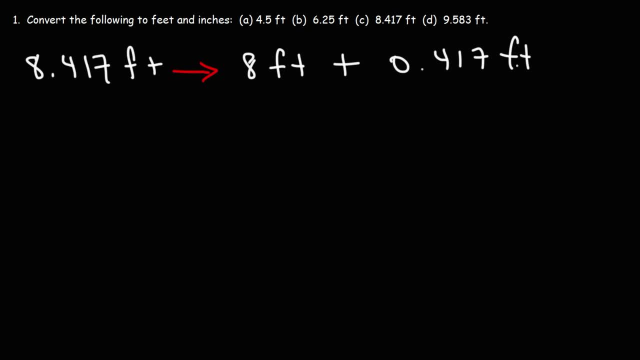 .417 feet. Now let's take the decimal part, the .417 feet, and let's convert it to inches, So, just like before, there's 12 inches in a foot. And let's multiply those two numbers .417 times 12.. This is 5.004, but we can say it's approximately 5 inches. 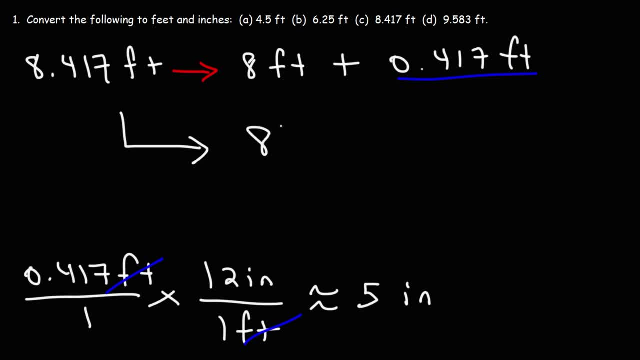 So our final answer is approximately 8 feet and 5 inches. Now let's do the same for part D. So we have 9.583 feet. Let's convert that. Let's focus on the decimal portion. We're going to multiply this by 12.. 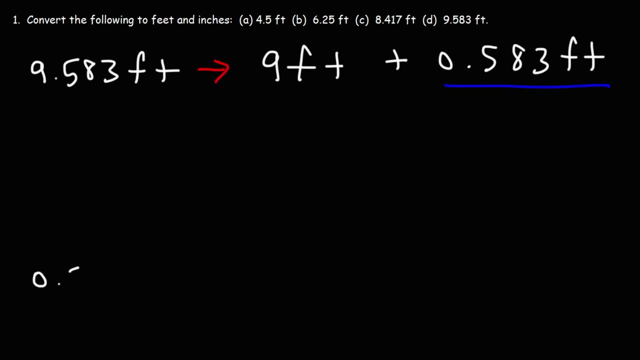